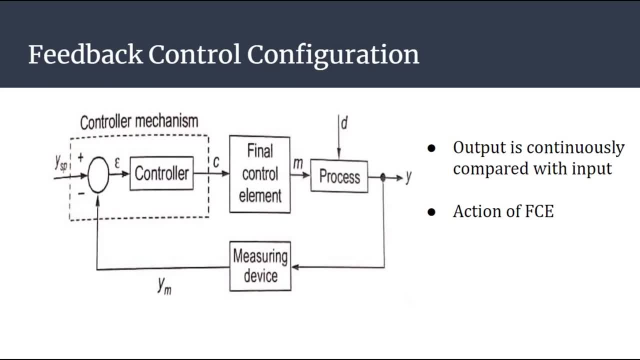 then tries to bring back the process to the desired level with the help of the final control element, Now controller control action to provide karega. Lekin wo jo control action provide karega? wo kaunsa cheez hai jo is control action ko actually like it will bring? 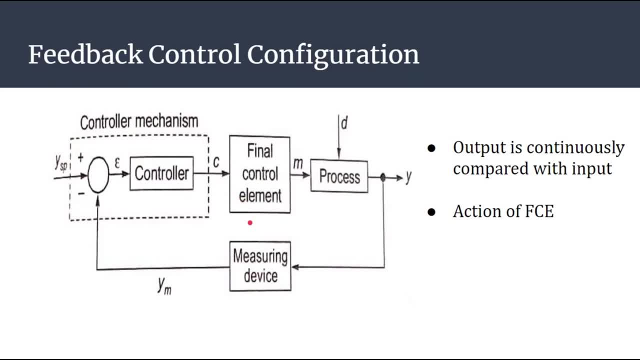 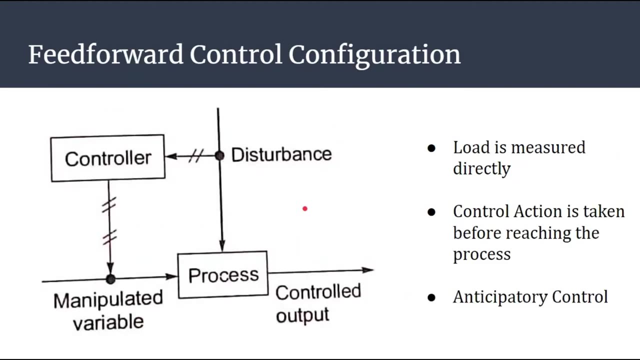 it to happen. This thing is our final control element, right? So final control element: ke zariye. Now controller control action process: pe provide karega. Okay, so this is all about our feedback control configuration. Now let us move to feed forward control configuration. So a feed. 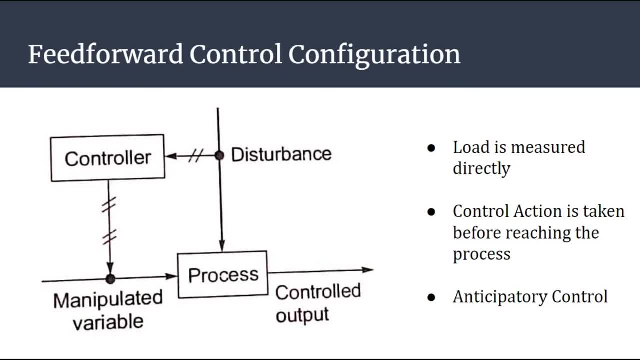 forward control configuration measures the disturbance or the load directly and takes the control action to eliminate its impact on the process. output Load ko siddha: measure kar leka and it takes the control action to eliminate the effect of disturbance. Okay now, this is the figure showing the feed forward control configuration And, in case of a feed, 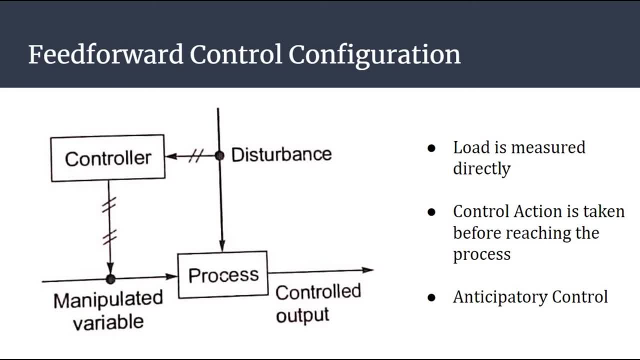 forward control configuration. the load will be measured directly and the feedback will be measured to eliminate the effect of disturbance. So this is the figure showing the feed forward control configuration. The effect of the disturbance is completely eliminated as it is already sensed and corrected before reaching the process. So process, reach karne se pehle hi control action. 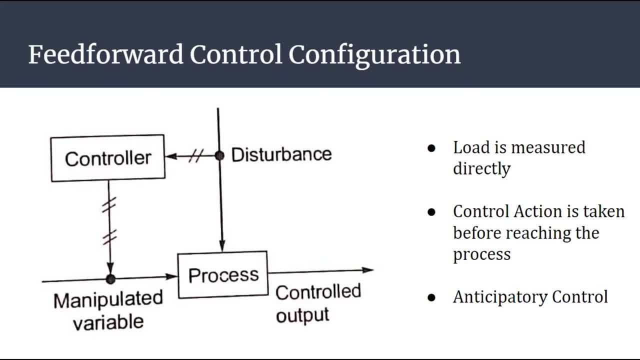 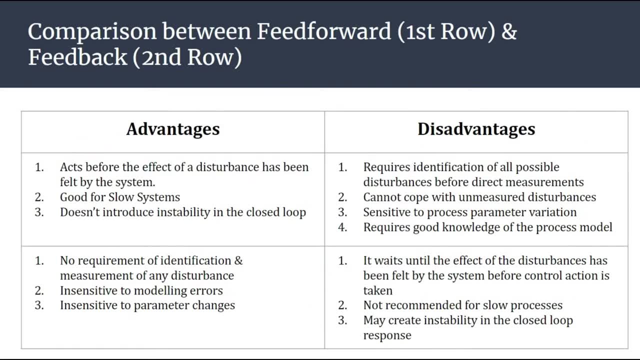 liya jata hai. This feed forward control acts beforehand, and it is also known as anticipatory control. right Now, since we are done with the feed forward and feedback control, let us compare both of them. I will compare the advantages and disadvantages. The first row: will be basically our feed forward control configuration. Now, since we are done with the feed forward and feedback control, let us compare both of them. I will compare the feed forward control configuration in a lineichen. and final, Let us consider this three Porsche. 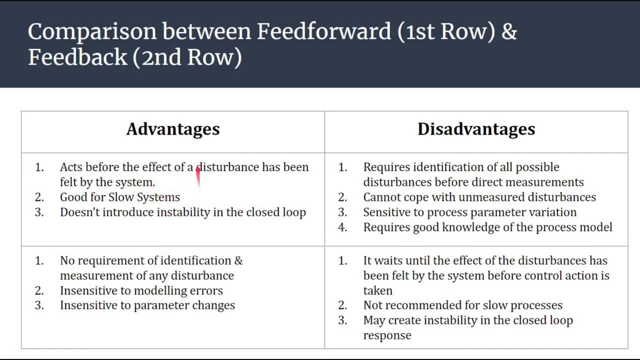 rivals. These three will be advantages of feed forward control configuration. These will be the disadvantages of feedback. This four will be the disadvantages of feed forward control configuration. And finally, these three writing will be the disadvantages of feedback control configuration. So at first let us go through the advantages of feed forward. control configuration. So feed forward. control configuration, as we know, is a saddle greener set type eyebrows, So you can see how the bold Techn Dodger move from merge stressed to max high to any specific perfectly at this position. Now, what all bad responsibilities. 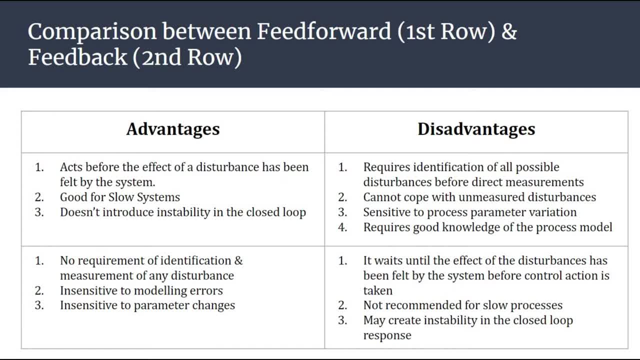 are at this point, sir. First, if associated with feed prioritization and anaesthetics, that it acts before the effect of a disturbance has been felt by the system- right. so it is good for slow systems or systems with significant dead time, right, and it does not introduce instability. 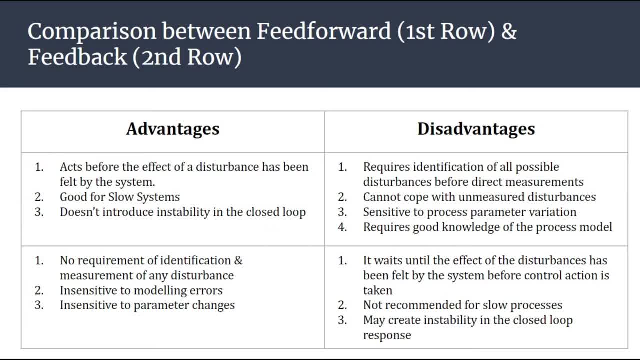 in the closed loop feedback ke baad karte hai. feedback ka kya advantage hai? there is no requirement of identification and measurement of any disturbance. right, yahi same cheez apna feed forward ka. feed forward control configuration ka disadvantage hai? feed forward- anticipatory action. 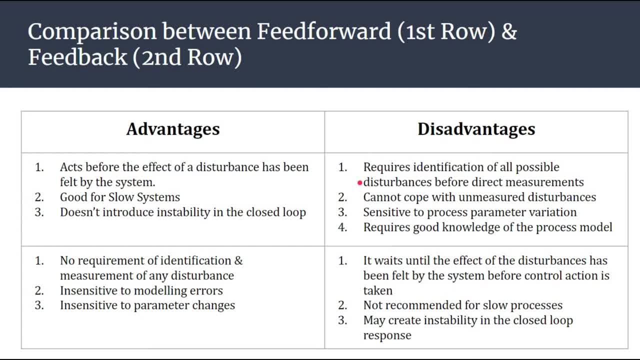 toh leh raha hai, lekin it requires identification of all possible disturbances before the direct measurement. lekin feedback pe aisa nahi hai, so that this particular thing acts as an advantage for the feedback control configuration. there is no requirement of identification and measurement. 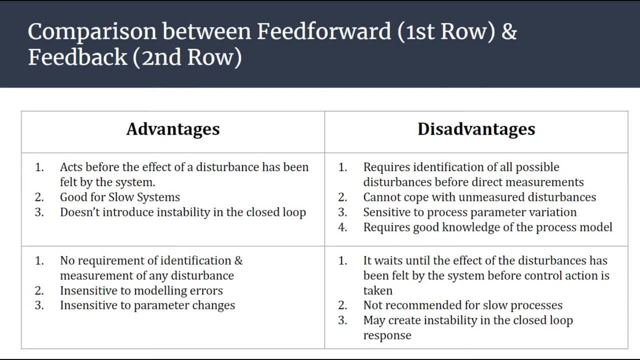 of any disturbance right feed forward ka ekor disadvantage hai. it cannot cope with unmeasured disturbance. jo disturbances ko feed forward, measure karega, wo feed forward, usi disturbance ke sath cope up karega, lekin jo disturbances, wo measure nahi kar paega, it cannot cope up with them. okay feedback is. 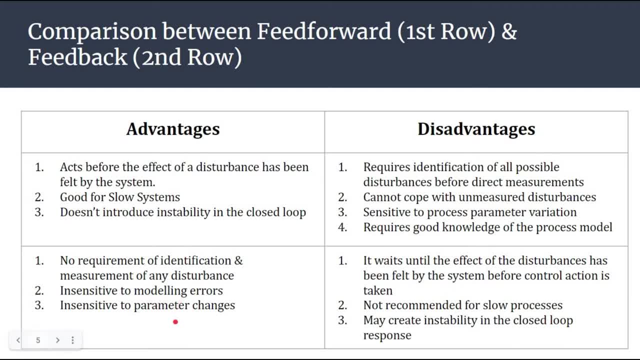 insensitive to modeling errors and insensitive to parameter changes. right, this is the advantage of feedback. but feed forward is sensitive to process parameter variation and in order to make a feed forward control configuration feasible, we require good knowledge of the process model. right now, let us go through the disadvantages of feedback control configuration. 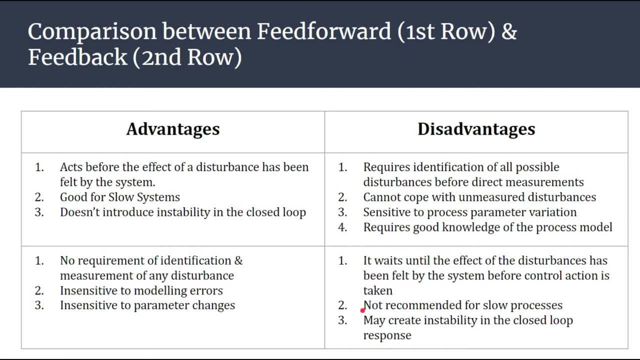 feedback control configuration is not recommended for slow processes or processes with significant dead time. it may create instability in the closed loop response. lekin this particular point is an advantage for feed forward, as you have already seen right. feed forward does not introduce instability in the closed loop, but feedback may create instability in the closed loop response. 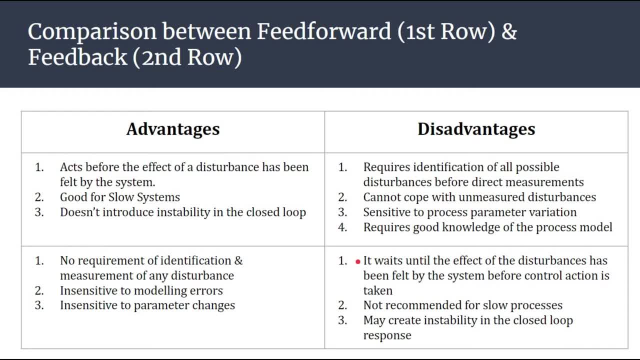 feedback also waits until the effect of the disturbance has been felt by the system before control action is taken. so disturbance ka effect is felt by the system before control action is taken. so disturbance ka effect feel, hone tak feed forward. wait nahi karega, wo already control action de de. 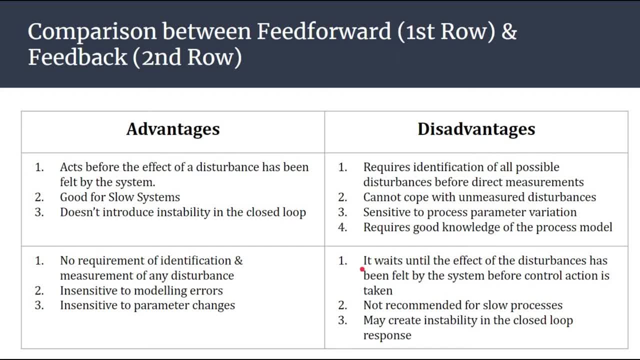 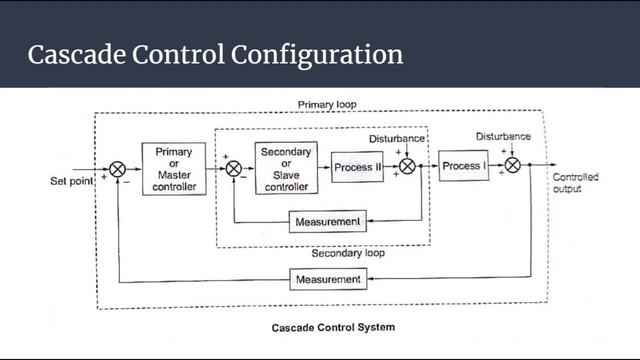 lekin feedback wait, karega, and this is the disadvantage of feedback right now, since we are done comparing our feed forward and feedback control configuration, let us go to cascade control configuration. so in cascade control configuration, as you can see, there will be one manipulated variable and more than one measurements. right, more than one measurement. 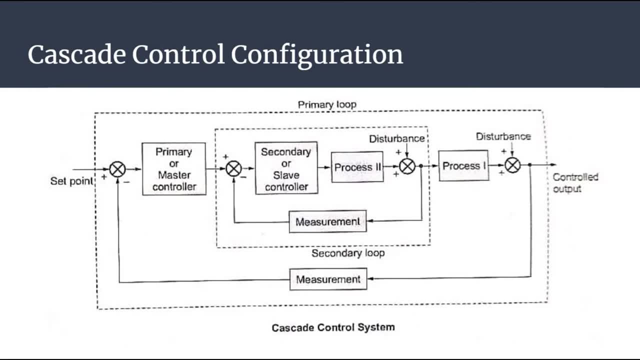 one measurement. an intermediate process variable that responds both to the manipulated variable and to some disturbances can be used to achieve more effective control over the primary process variable means. by introducing secondary and slave controller, we are creating an intermediate process variable that can respond both to the manipulated variable and to some disturbances. 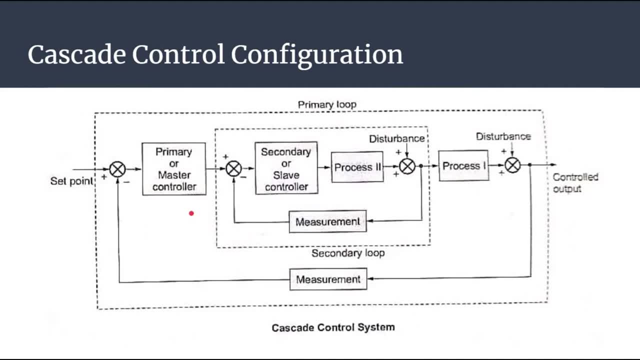 right. first we had a primary and master controller, but by using secondary and slave controller we are introducing this particular advantage in our cascade control configuration. now the cascade loop consists of two or more controllers in series. as you can see, the master controller, as in, is in series with the slave controller, right, but only have a single. 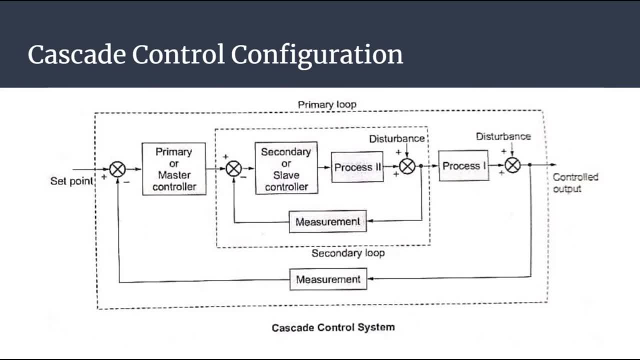 independently adjustable set point by the operator to the master or the primary controller, though the controller is with the cascade control configuration. but we have only one set point, and this is an independently adjustable set point by the operator to the master or primary controller. it will not go directly to the secondary or slave controller. right now, the use of secondary 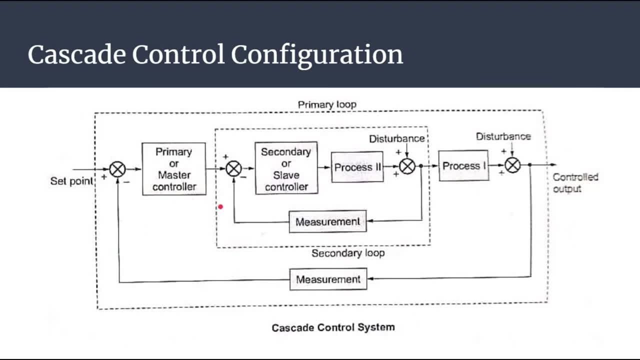 or slave controller whose set point is determined from the output of the master controller. output is basically the input or the set point to the secondary or the slave controller. right now, that what is the use of secondary or slave controller? then it is to act as the first line. 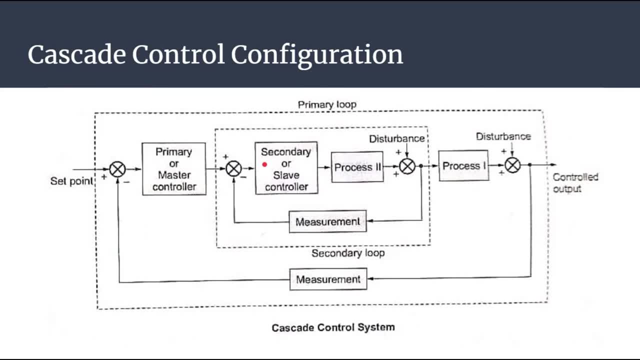 of defense against disturbances, a set point for givenポitions, Preventing these upsets from entering the primary process. Who will deal with disturbance? Secondary and slave controller? Who will save the process of primary and master controller? The secondary loop must have faster dynamics than the primary loop for the cascading effect to yield better results. 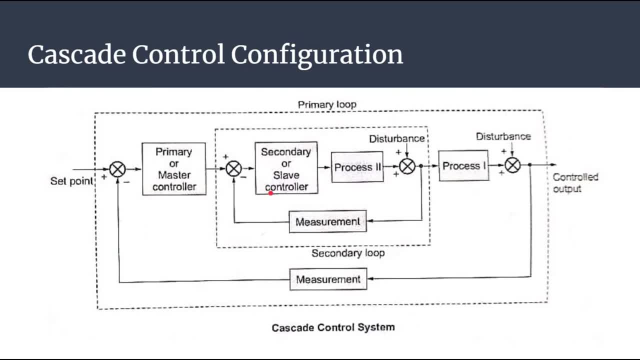 Whose dynamics should be faster- Secondary and slave controller- So that they can save the primary controller from the effects of disturbance. Now there are two interesting points about the cascade control configuration. So in cascade control configuration the crossover frequency for the secondary or slave loop is higher than that of the primary loop.